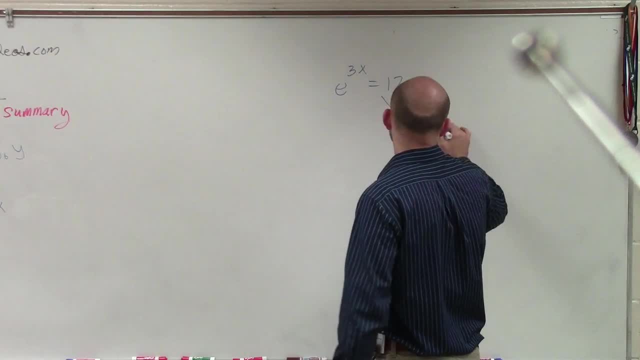 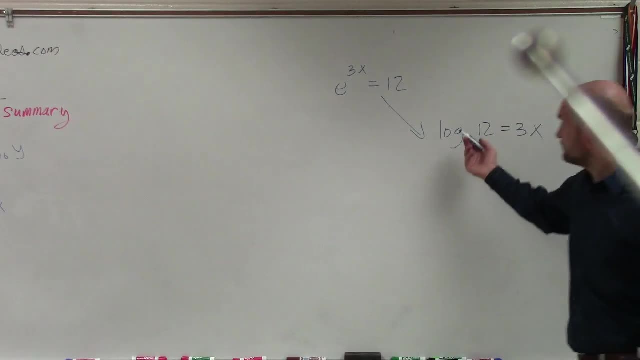 up into the power. But if I rewrite this in exponential form, this is now going to be log base e of 12 equals 3x. Now, remember, we write log base e of 12 as ln of 12 equals 3x. So now, 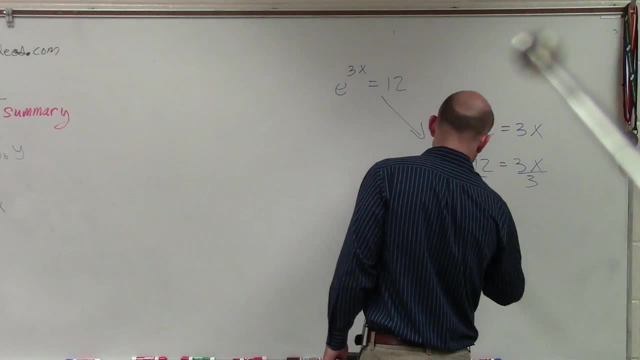 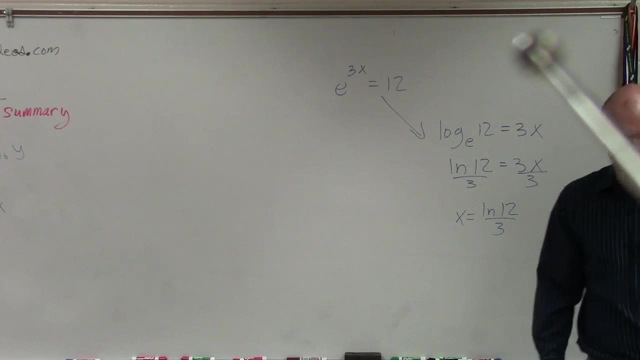 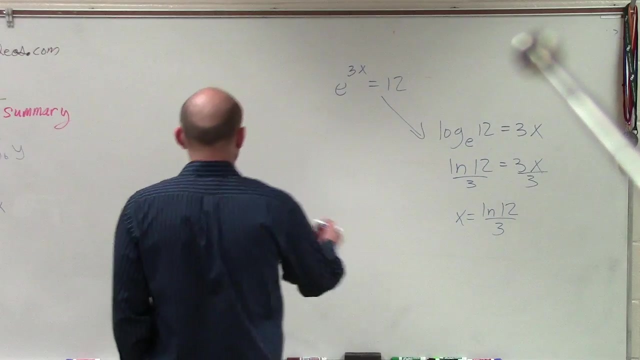 to solve for x, you divide by 3.. So x equals ln base 12 of 3.. Okay, Now, that's one way you guys can go ahead and do this. The other way that you can look at this is again by taking the. 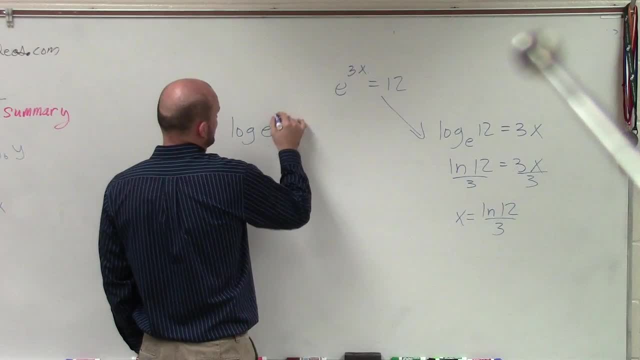 log base e of 12, as ln of 12 equals 3x. So now to solve for x, you divide by 3.. So x equals the log of both sides. Again, ladies and gentlemen, when we're looking at this- and let's 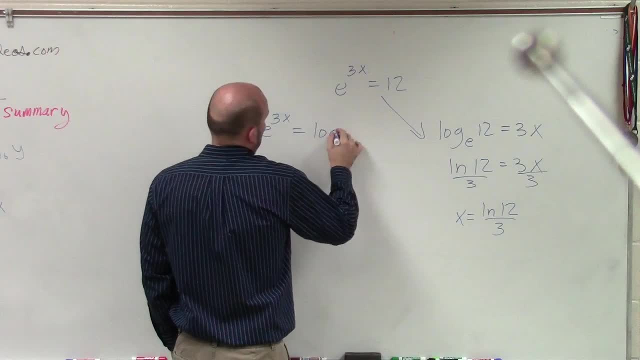 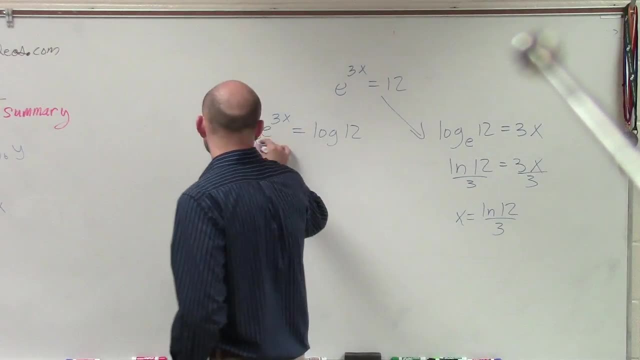 go to our properties of logs. Now, of course, ladies and gentlemen, I don't want to take the log of both sides because I need to choose a base. Remember, I kept on telling you the base has to be e right. You always want to have the base of your logarithm be the same base of your 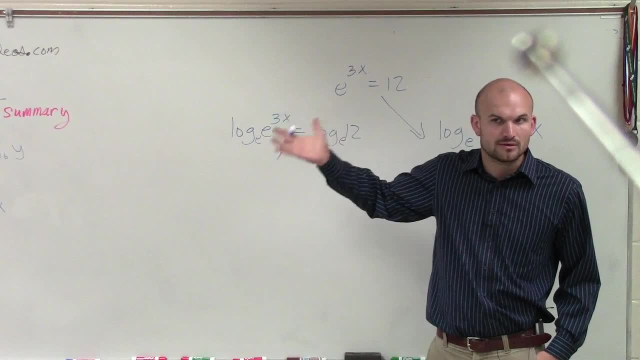 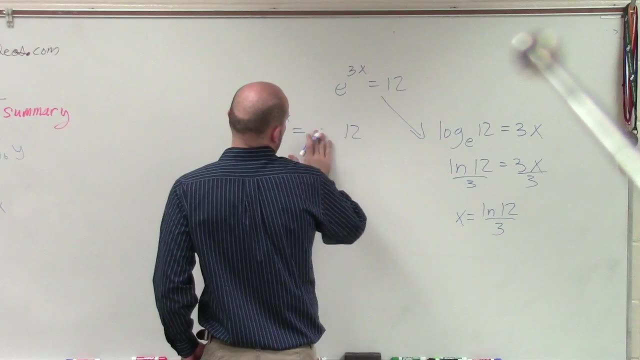 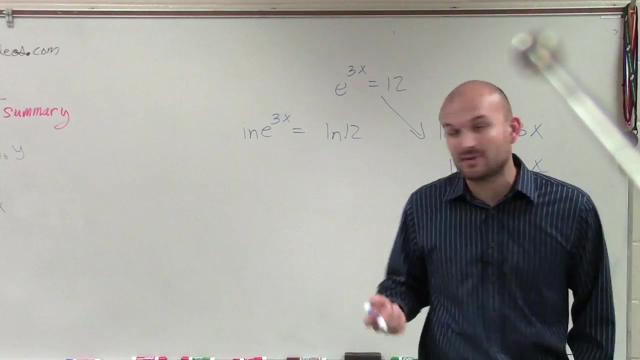 exponent. Well, log base e is what we call, what ln. So let's just take the ln of both sides Now, by applying the properties of logarithms. maybe this will make a little bit more sense for some of you If, by applying the properties of logarithms, we can take this exponent and put it: 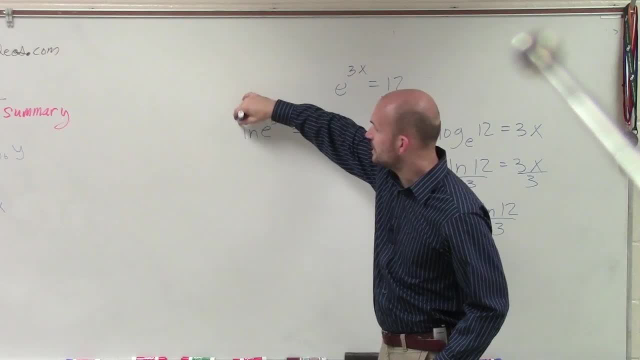 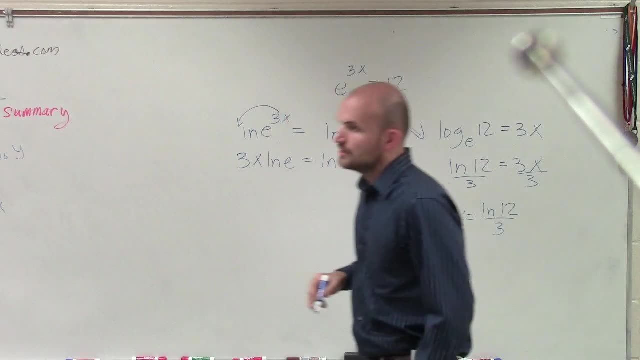 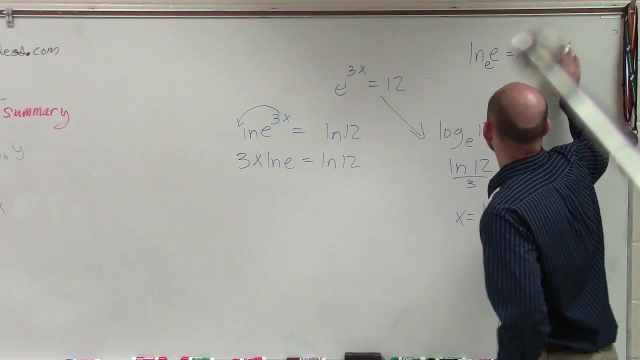 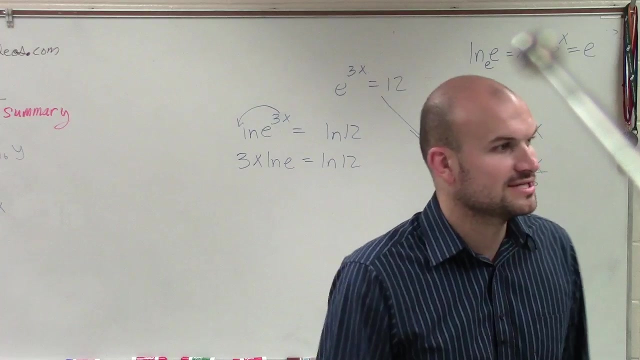 where In front right And write it as the product. So this is 3x times ln of e equals ln of 12.. Now let's evaluate ln of e. So what that says is: e raised to what power equals e. e raised to what power equals e 1.. 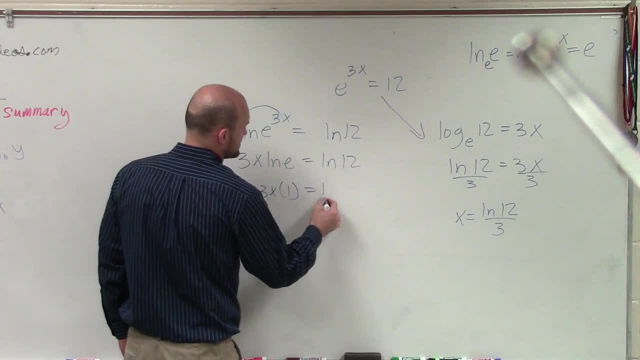 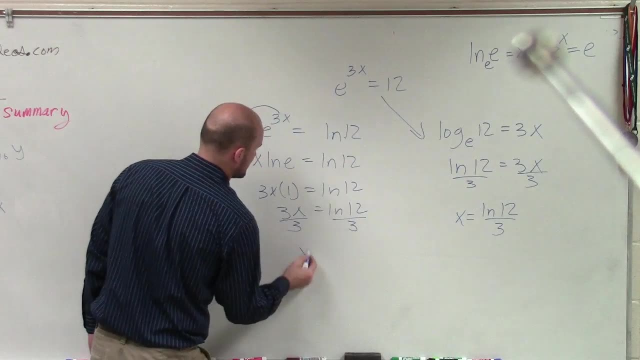 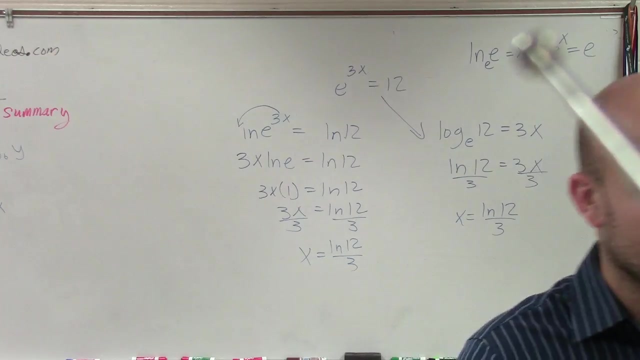 So guess what? It's just 3x times 1 equals ln of 12, or 3x equals ln of 12.. Divide by 3, divide by 3, x equals ln of 12, divide by 3.. You're getting the exact same answer, But now. 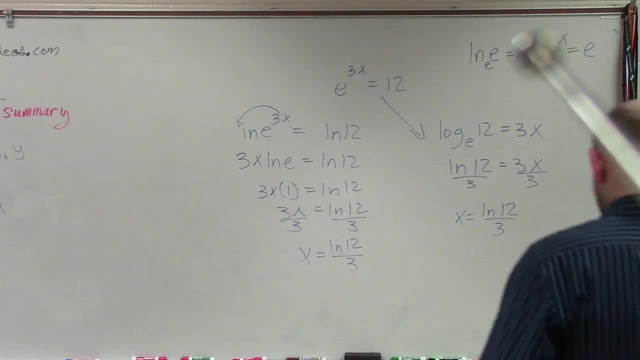 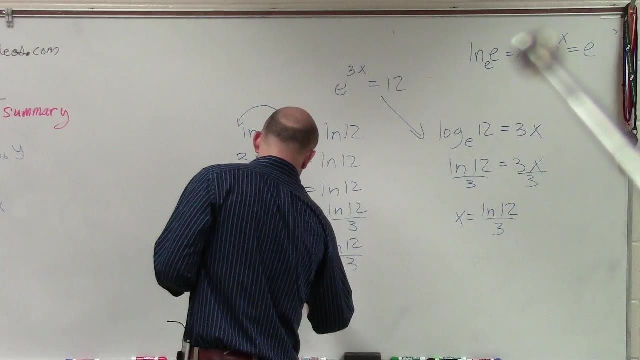 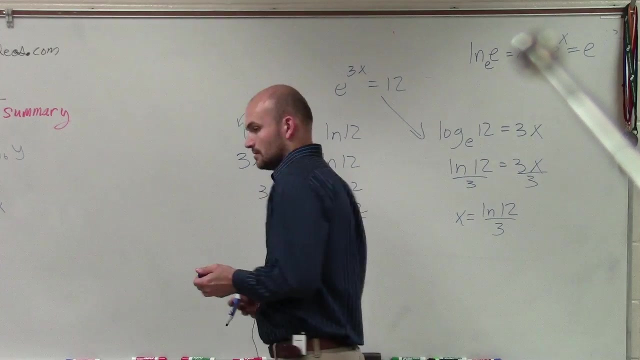 what we need to do is Solve this So we can go in our calculator and we type in ln of 12, and then we divide that by 3.. So therefore, x equals 0.83,, approximately because we're buying- Okay, Anybody have any.